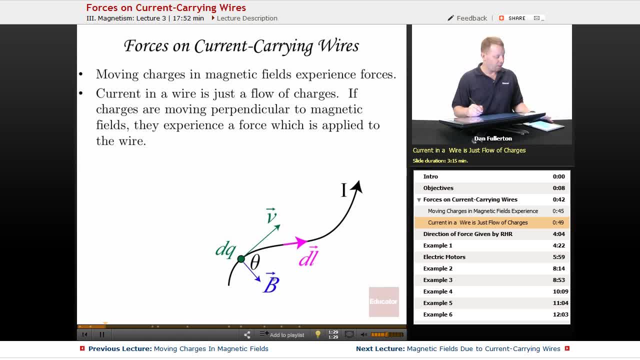 our magnetic field is here in blue capital B. Well, in order to find the force, the magnetic force, what we're going to do is say that the magnetic force, FB, is equal to Q, v cross B. But since we're only looking at a very little bit of charge, let's look at the tiny bit of force. 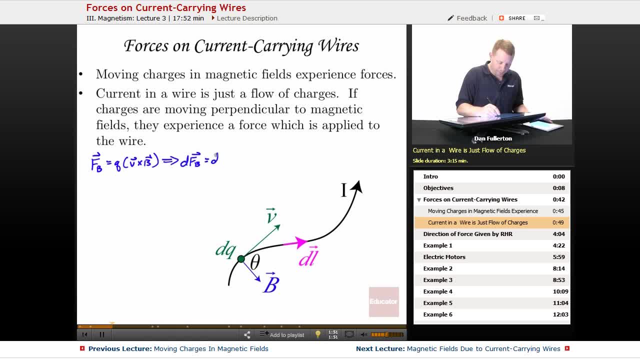 The differential of the magnetic force then will be dQ, v cross B. That little bit of charge, its velocity crossed with the magnetic field at that point. This implies, then, that the magnetic force is well, let's take a look here. 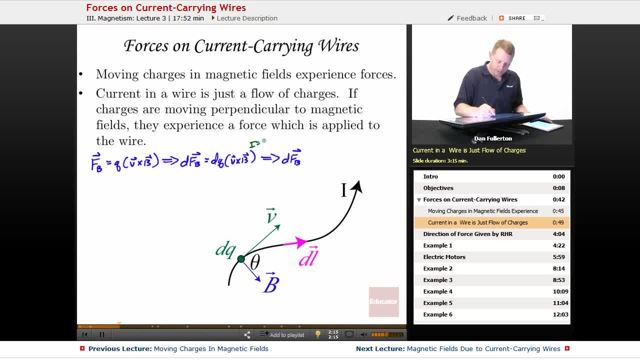 If we think of it as current, being equal to dQ, dt. dQ we could write as I dt, So the magnetic force is equal to. we'll replace dQ with I dt times v cross B, But we also know that v is dL, dt. 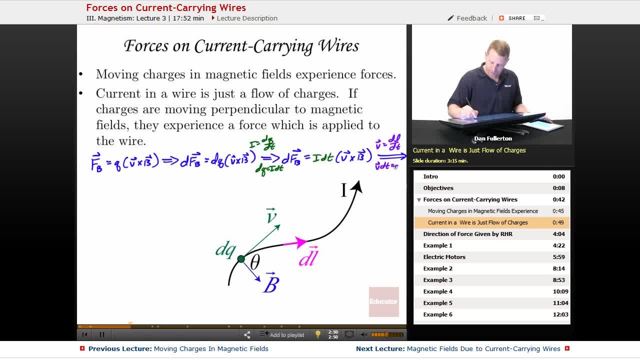 Therefore, v dt must be dL, So we can now write this as the dL dt. So we can now write this: as the differential of that magnetic force is equal to. we have our I. we have. well, v dt we said was going to be dL. 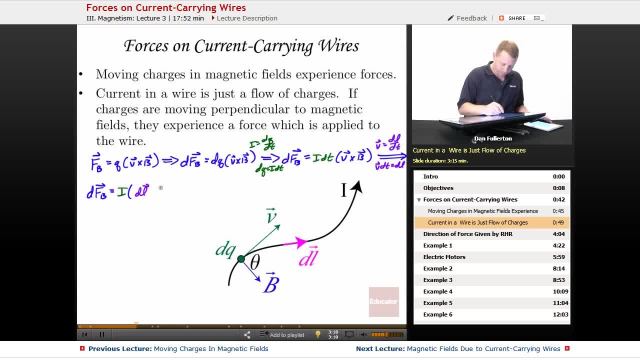 so that will be dL crossed with B, Or taking the integral to get the whole thing. the integral of dFB is going to be the integral of I, dL crossed with B. The integral of the differential of the magnetic force is going to give you the entire magnetic force. 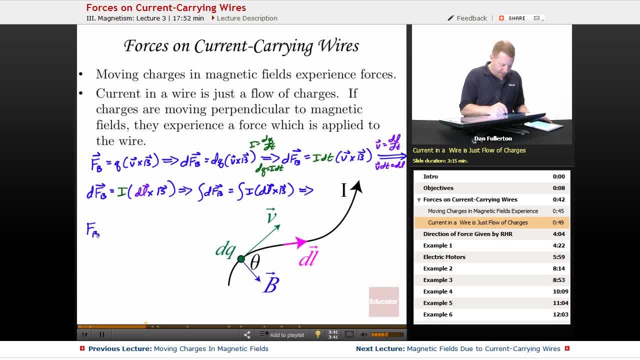 So, to finish this up, the magnetic force is going to be the integral of the current times. dL crossed with the magnetic field B, So that's how we can find the force on a current carrying wire due to a perpendicular magnetic field.